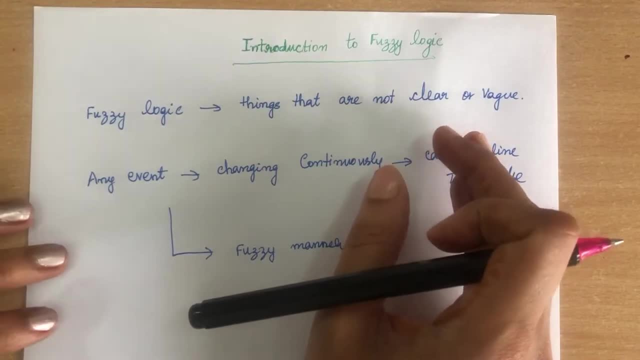 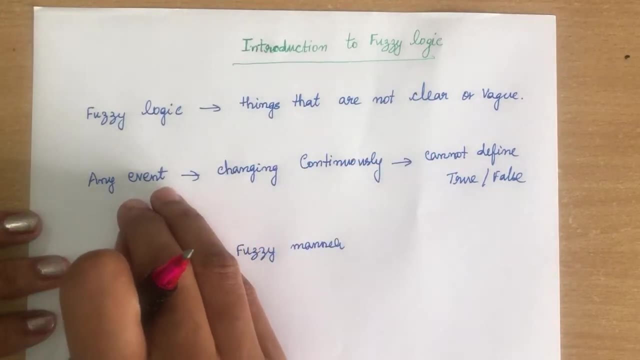 if a problem is not clear, or if it is vague, or if it is not precise or ambiguous, then we can able to solve that problems using fussy logic. So I can tell you one more example. like any event, if it is changing continuously, we cannot come to a conclusion. whether it 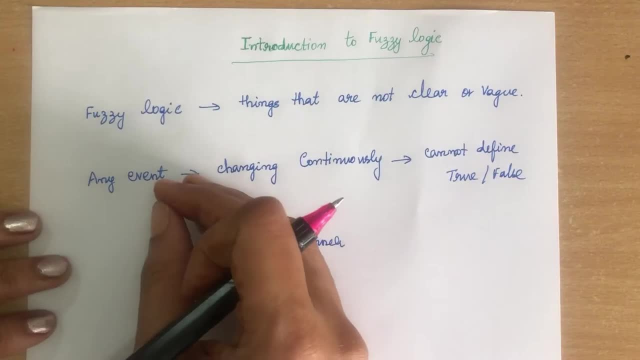 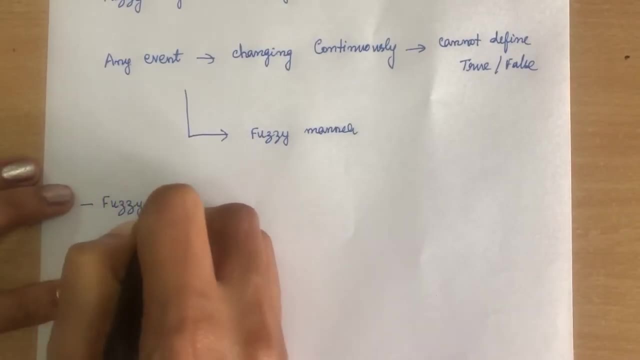 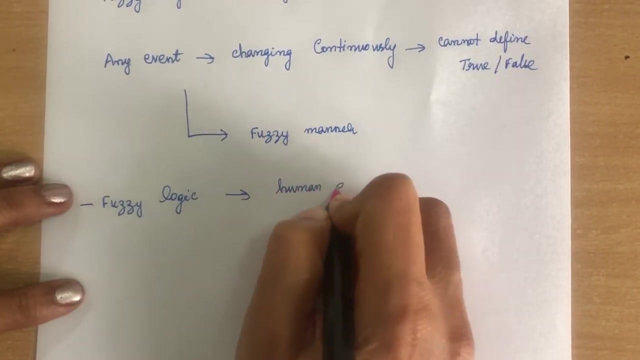 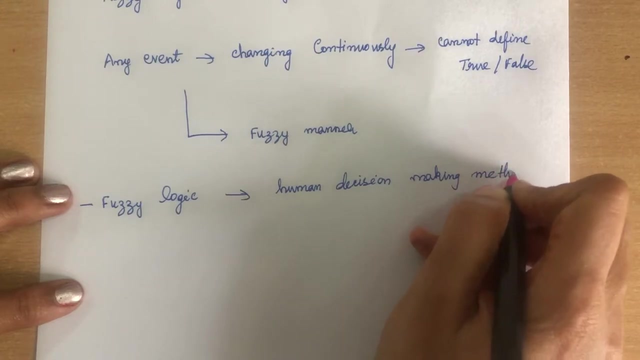 is true or false or we cannot conclude anything, then we can solve those problems using fussy logic. So fussy logic, it resembles fussy logic, it resembles human decision making, metrology. So how human thinks. So we are going to solve the problems using human decision making. 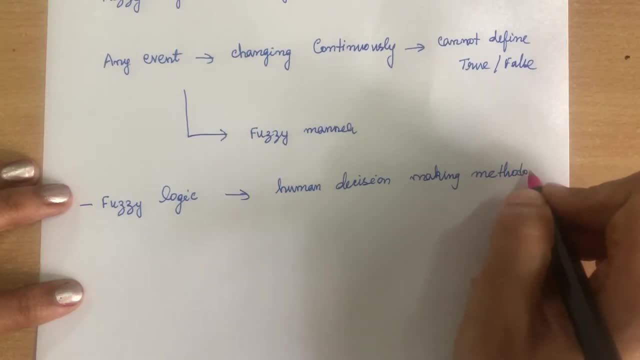 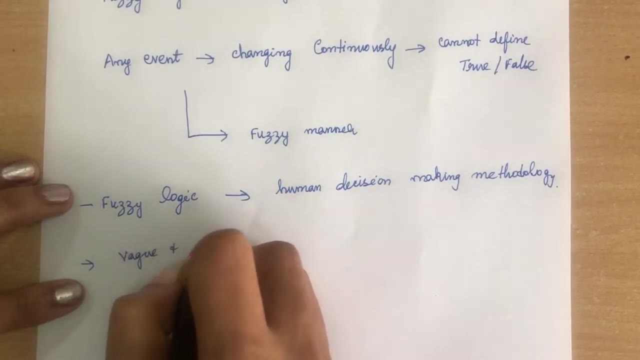 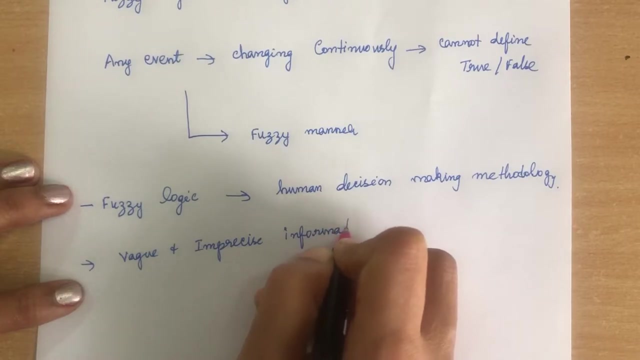 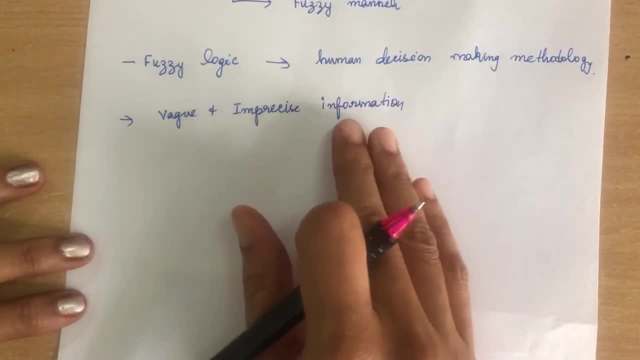 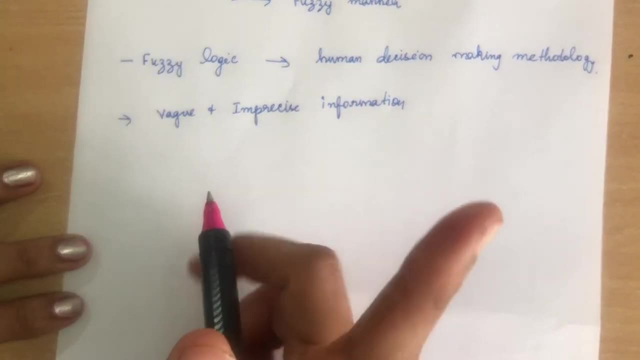 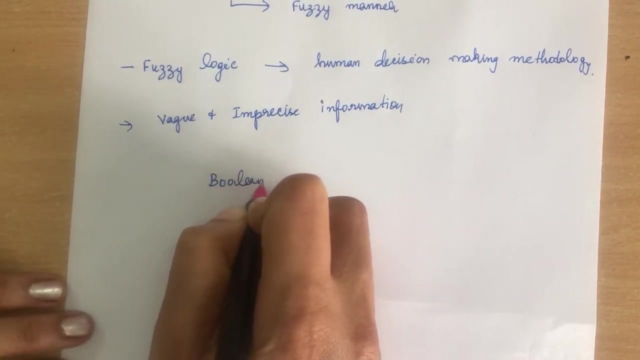 If the information is incomplete, then we can able to easily solve those problems using fussy logic. Now let me tell you the difference between two logic. So we know there are two logic available. One is the previous existing logic is Boolean logic. It is called as Boolean logic. 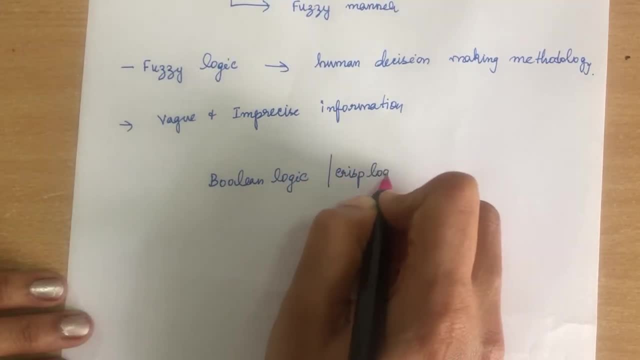 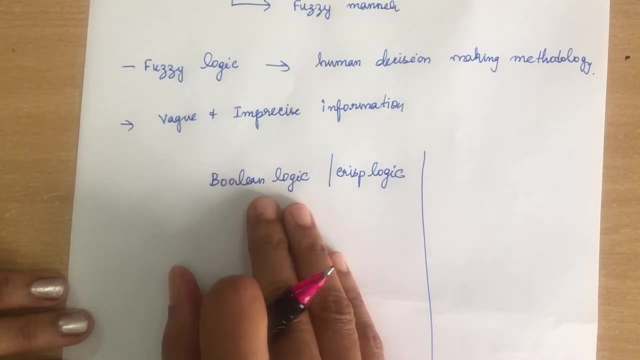 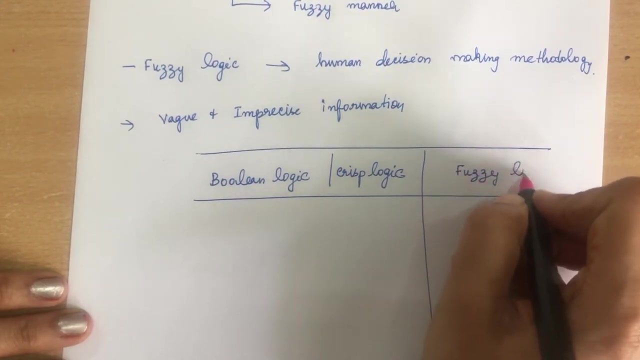 or otherwise, we can call it as crisp logic. So this is the logic which was existing, like mathematical, all mathematical functions. we will be solving it using fussy logic. One more logic which came into existence is fussy logic. So now I will tell you the difference between Boolean logic and fussy logic. 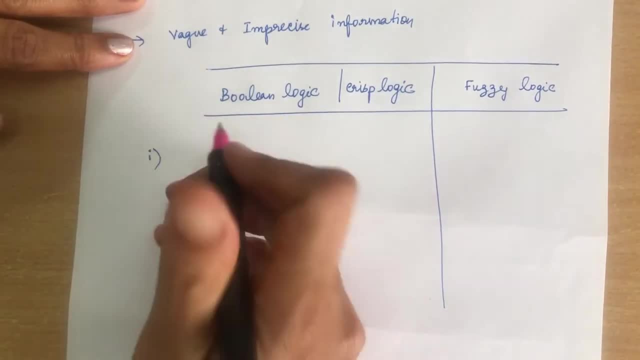 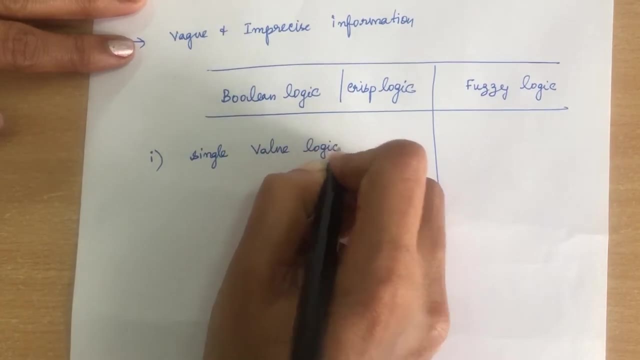 Coming to this difference. the first difference is Boolean logic. it will have only single value, So we can say: it is single value logic which can either it can be 0 or 1,, 0 or 1, or it can be true or false. 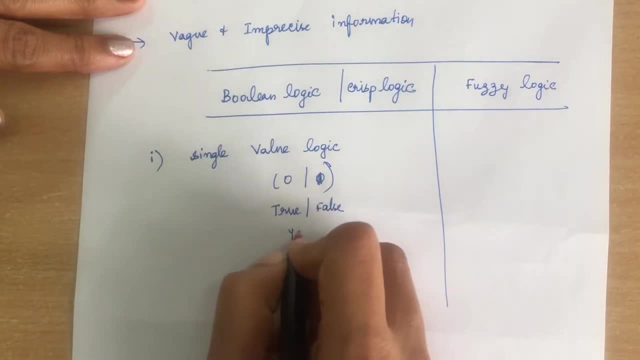 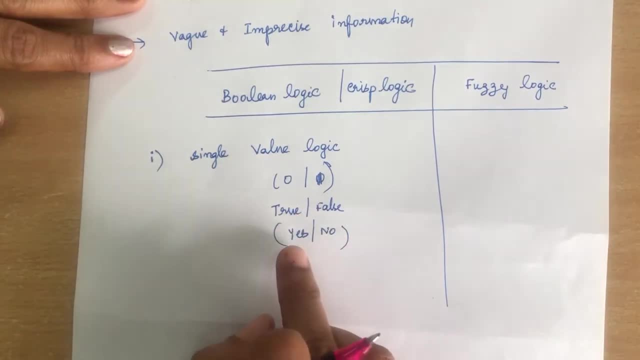 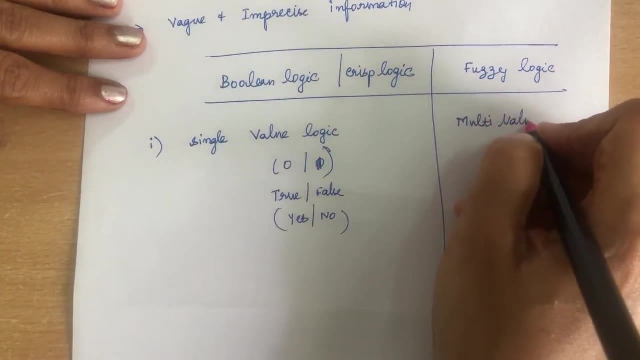 either it can be 0 or 1, it can be true or false, or it can be yes or no. Coming to this fussy logic, it is a multi-valued logic, So it will also have the values between 0 and 1, but it will not have two values. it. 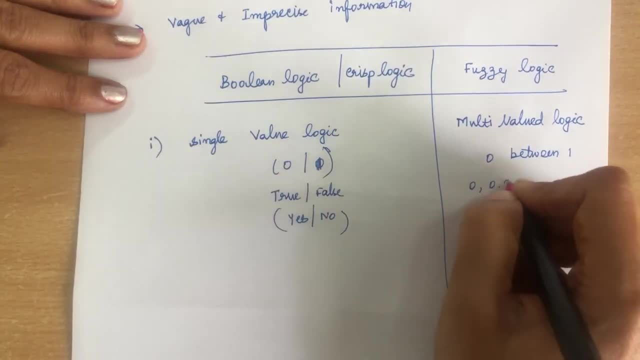 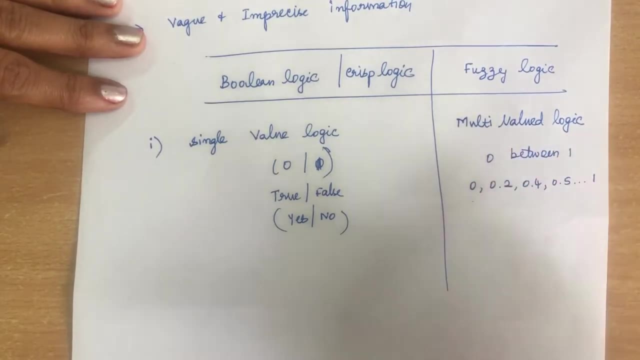 have single value like 0 or 1. It can be 0,, 0.2,, 0.4,, 0.5, any values between 0 and 1. So it is multi-valued logic. Next come to the second difference. So here it deals with all precise. 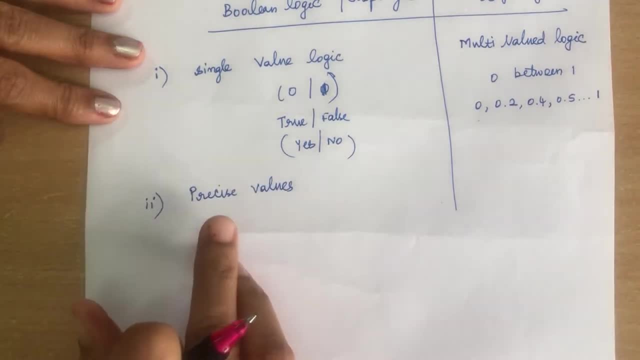 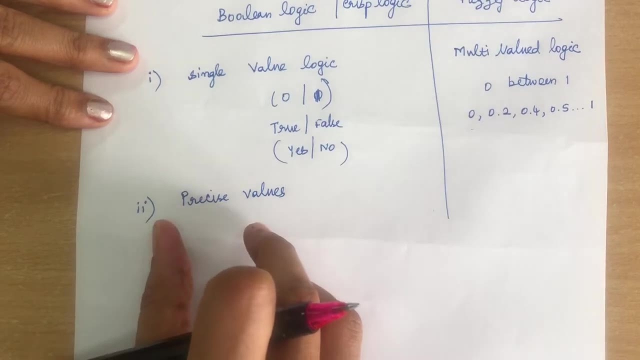 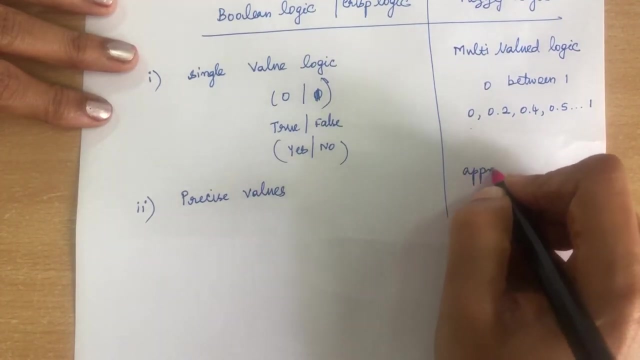 values. So if the problem is precise, if the problem contains all everything is correct, then we can solve it using Boolean logic. So the problem, if it is precise, then we can solve it using Boolean logic. Coming to this fussy logic, if the problem is approximate, If we can't solve, 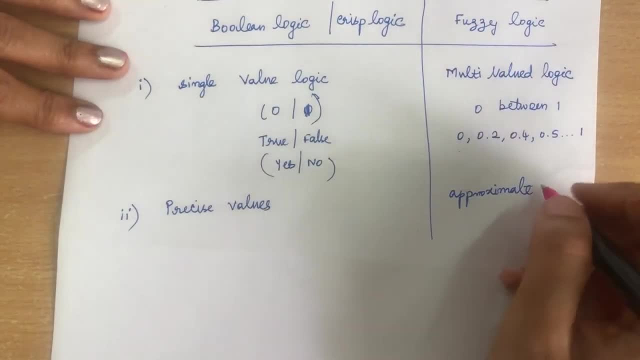 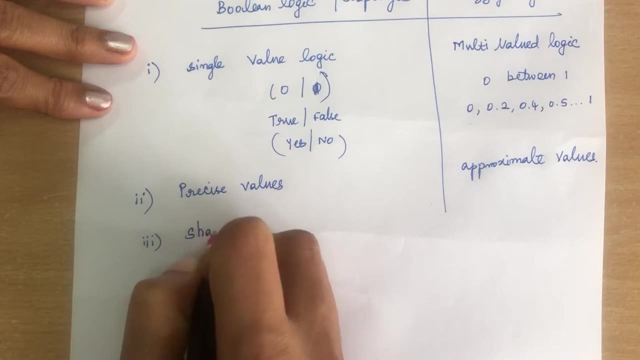 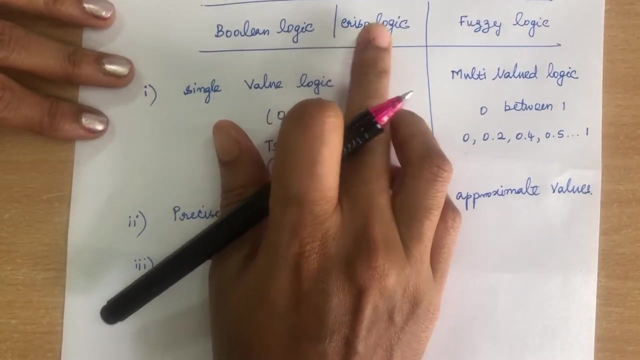 it by using Boolean logic, then we can solve it by fussy logic, So it deals with all approximate values. And third one: So here it will have all sharp distinction. So since it is very crisp, the name itself, it is crisp logic, So it will have a sharp boundaries, So it uses sharp 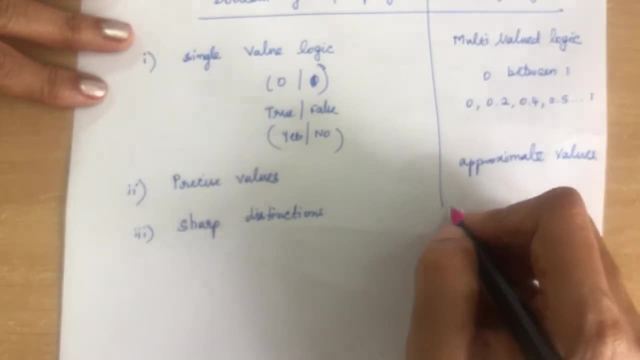 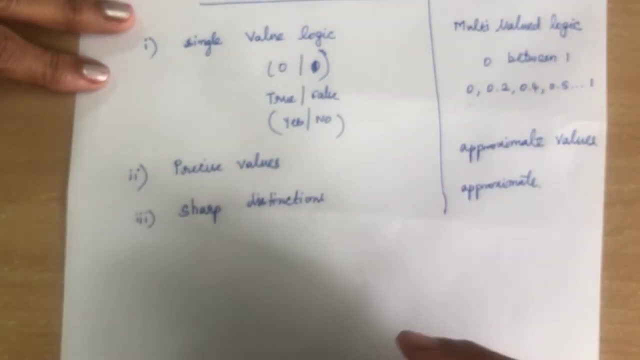 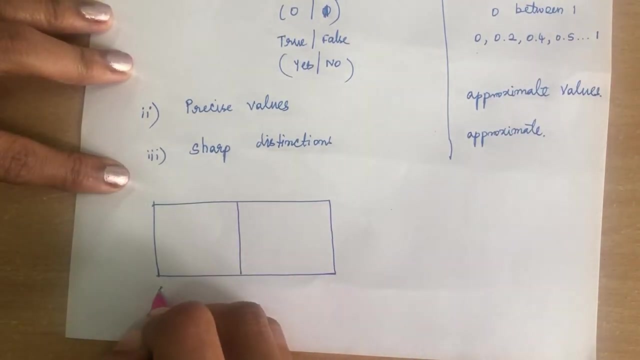 distinction To solve the problems. But here it will use approximate values. It is approximate, It uses how the people thinks. So the next is coming to the diagram. Here it will be. suppose you are having a value 0 here and 1.. So either it will be 0 or otherwise 1.. This is your Boolean logic. 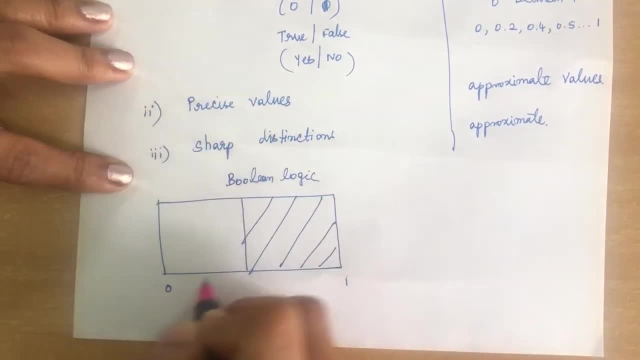 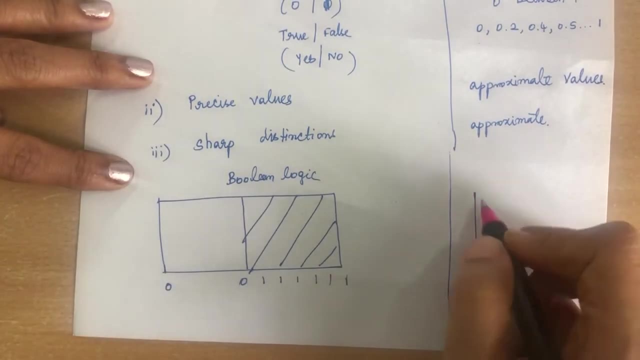 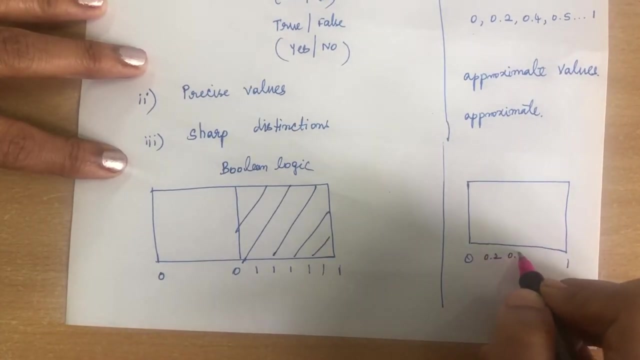 Ok, You will have the values 0 or otherwise. these all the values between 1.. But coming to the fussy logic, it can take a value between 0 and 1.. That is like it can take 0.2,, 0.3, 0.4, any values it can take from 0 and 1.. 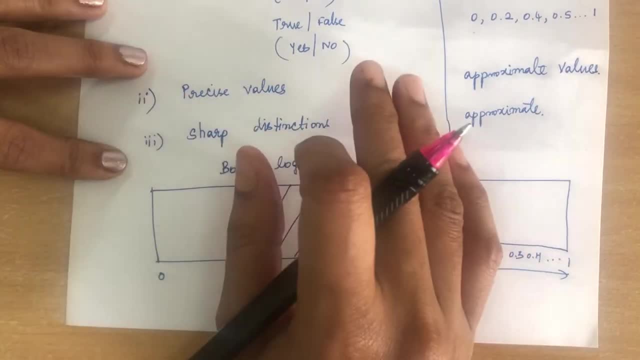 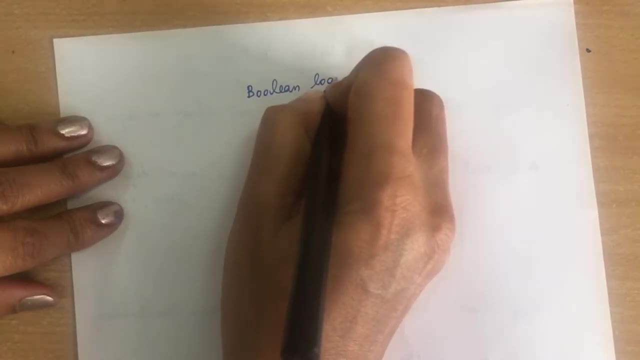 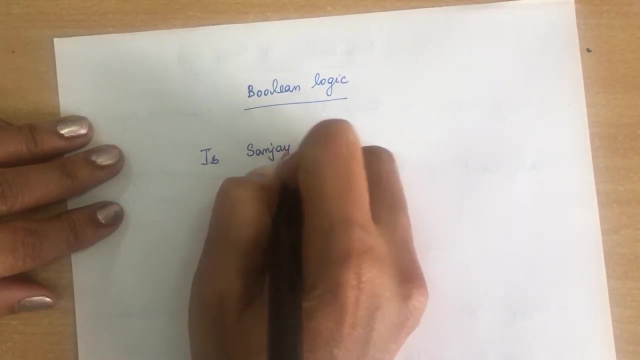 That is fussy logic. Let me explain this fussy logic in detail. Coming to this example, First let me explain this Boolean logic. So, coming to this Boolean logic, For example, I am having this example: like is Sanjay tall? Is Sanjay is tall? So if your are asking for a person to our parents, 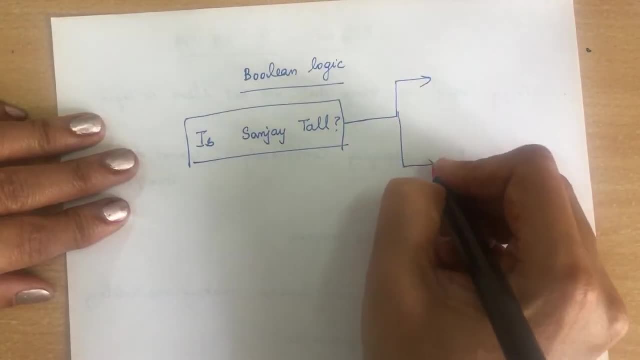 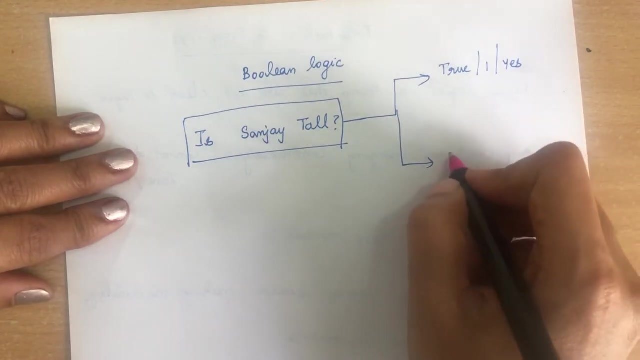 is Sanjay tall. so the parent is giving you the answer: either true or it may be 1, or it may be yes or here false, no, 0 or no, Everything the same over here. So either he can give true or false, 1 or 2.. 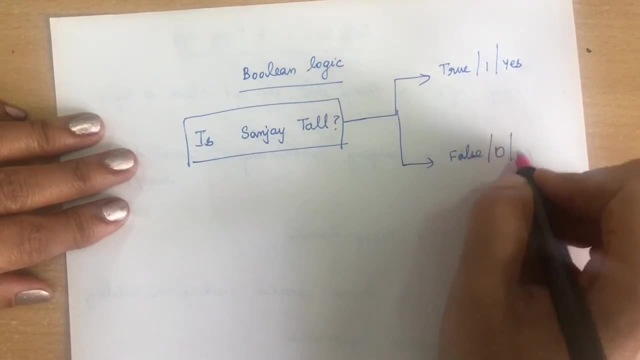 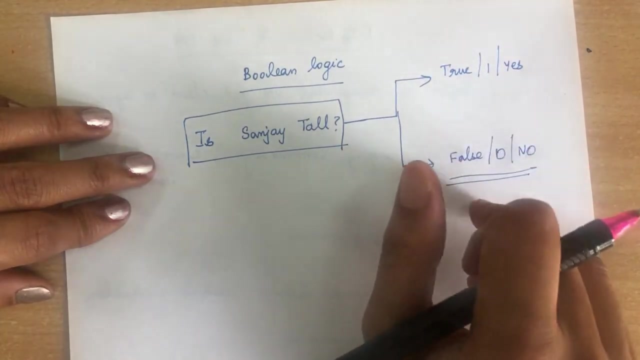 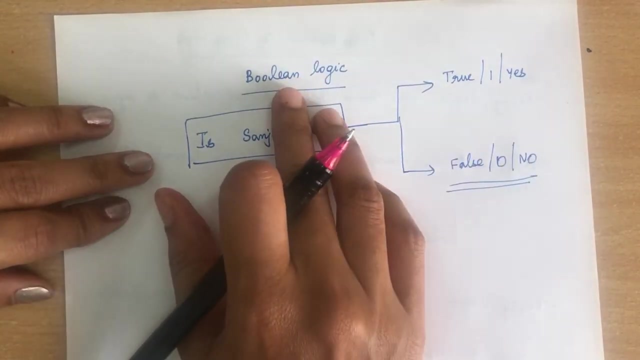 Ok, Its the same over here. So either he can give true or false, 1 or no, 2. So or 0 and yes or no. it contains only two values, either 1 or 0. so this type of problems are called. 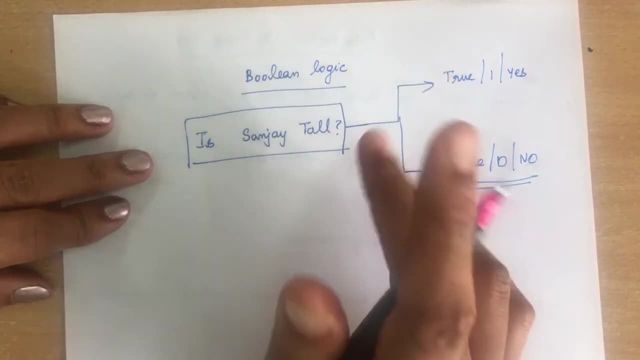 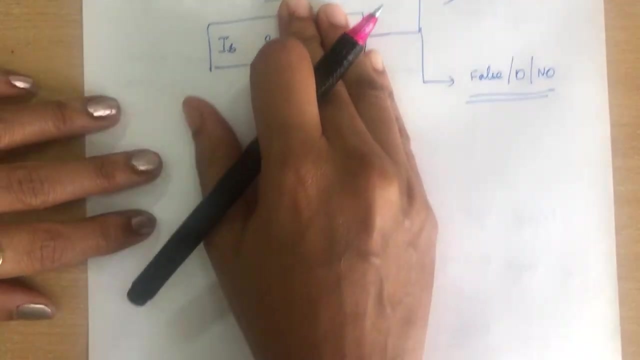 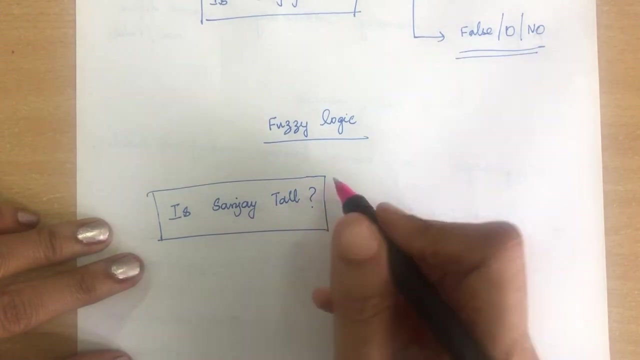 as Boolean logic. so you are giving to, you are going to give only one answer, either 1 or 0, that that example, those examples are called as Boolean logic. okay, now you are going to ask the same question to any other person. is Sanjay tall so he cannot able to give you the correct answer? 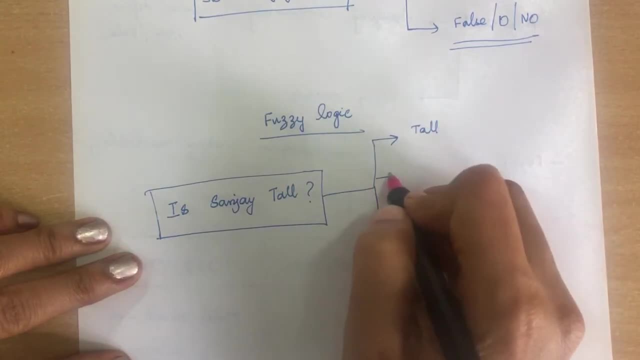 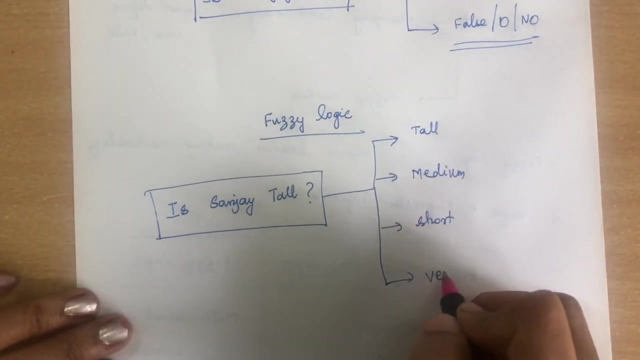 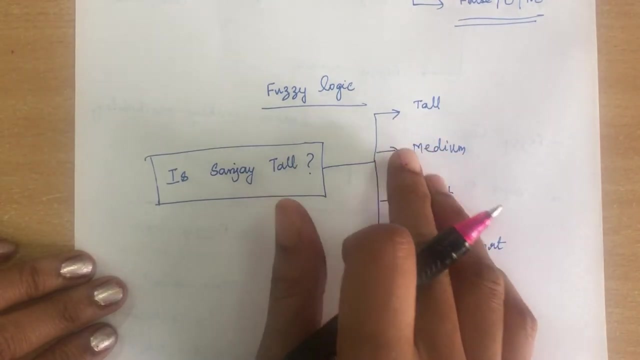 in that way he can tell that he may be tall, he may be medium or he may be short or he may be very short. so there are so many answers over here. so he we will classify into four types: tall, medium, short and very short. so we will give the values for this. short is represented by the 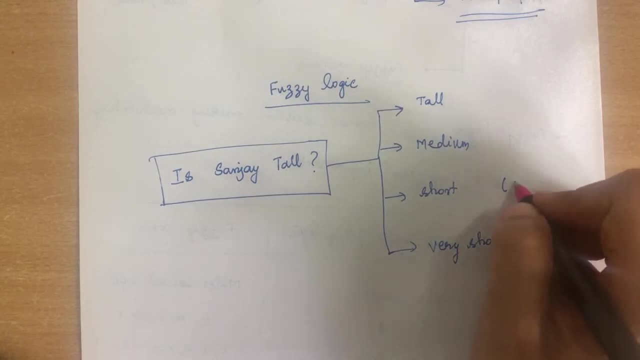 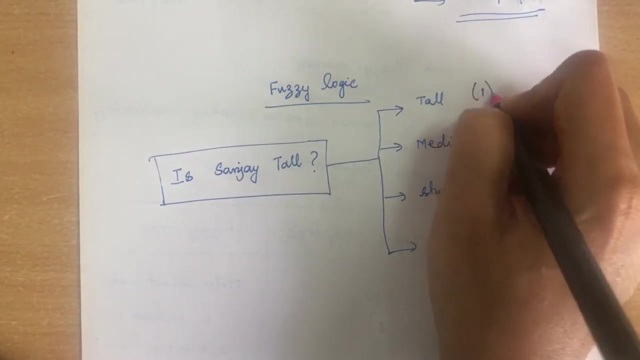 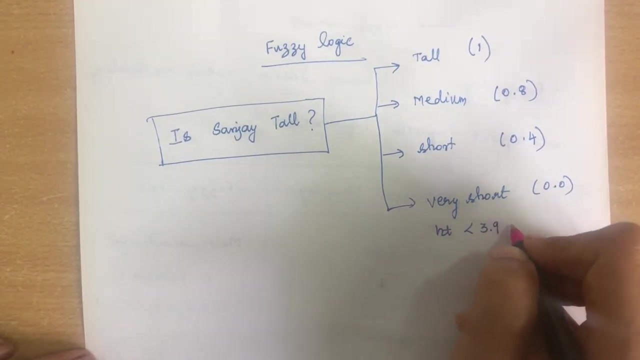 value 0.0 and for this very short. so for the short I am giving a value called 0.0 and for the medium I am giving 0.8 and for the tall I am giving the value 1. so, for example, if the person height is less than 3.9 feet, okay, I am, I am classifying it as very short. okay, I am. 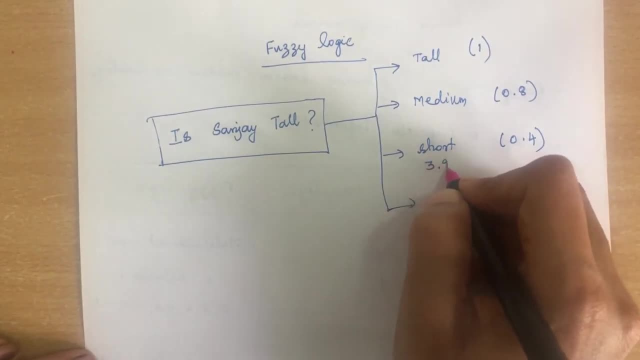 giving a value 0.0 if the person's height is 3.9 to 4.5- okay, 3.9 to 4.5 feet, I am classifying him as short person and I am giving a value 0.4- and if the person's height is less than 3.9 to 4.5. 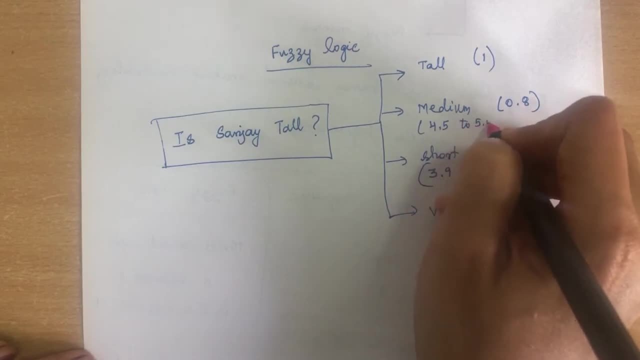 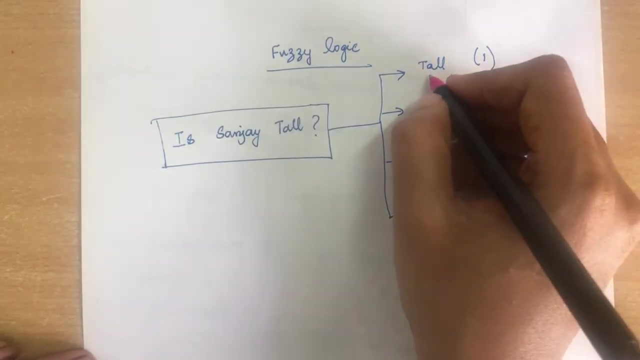 if the person's height is between 4.5 to 5.55 feet, then I am classifying him as medium person and I am giving a value called 0.8. if the person is above 5.5 feet, then I am classifying him as. 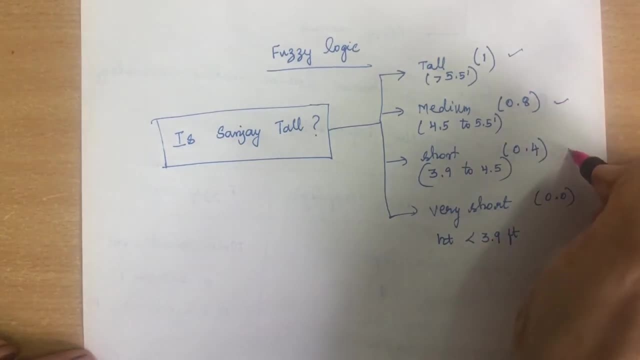 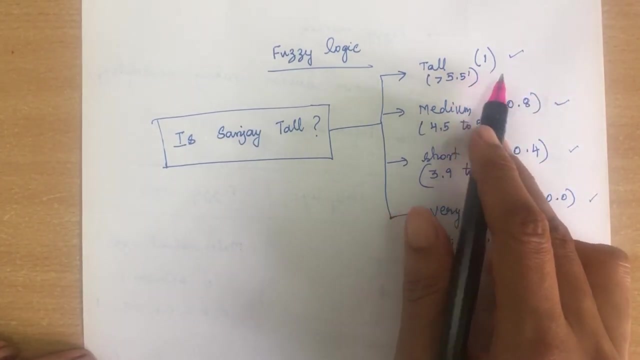 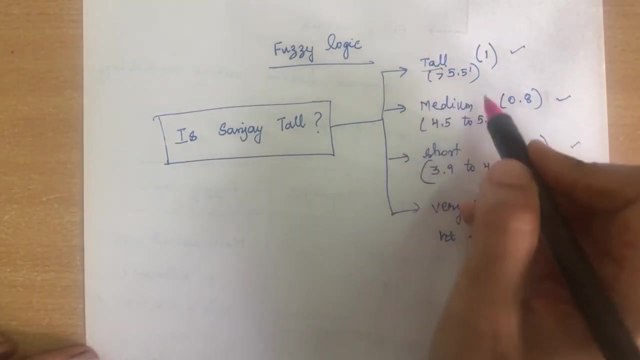 tall person. so here you can see I don't have only one value, 0 or 1, I am having multiple values over here. I can give them numbers, different values between 0 and 1, based on these variables. so I can call these variables tall, medium, short, very short. 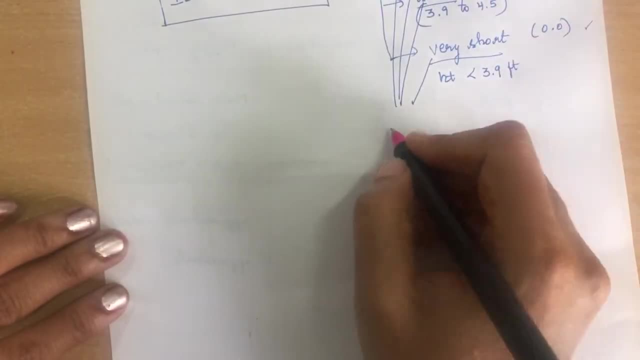 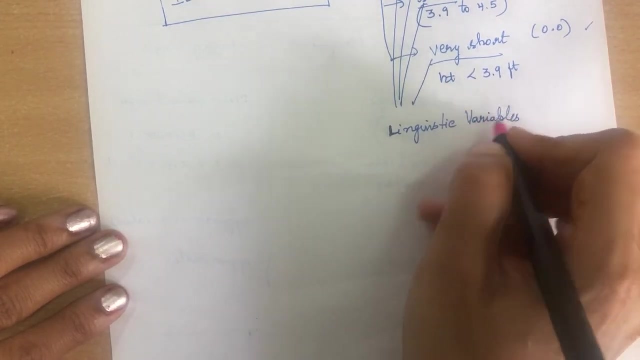 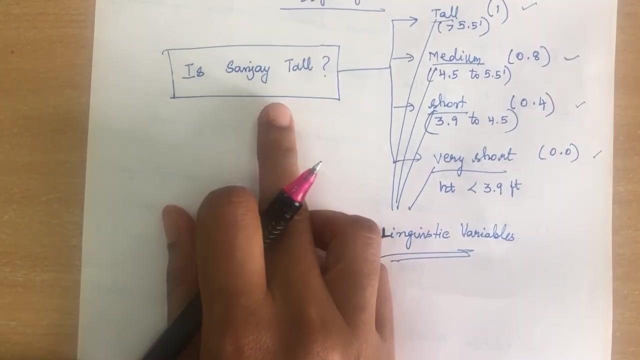 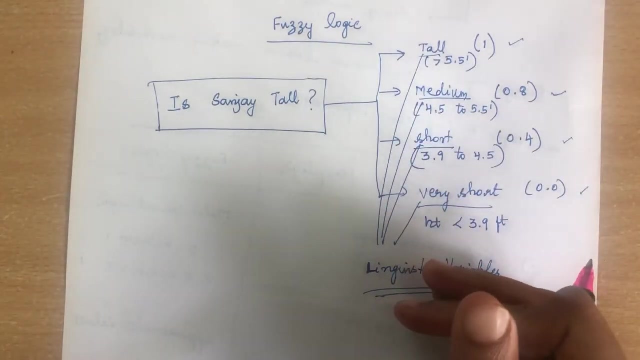 all these variables are called as linguistic variables. okay, these variables are called as linguistic variables in fuzzy logic. so how you are going to solve the problem? if you can't able to tell the correct answer, then you are going to classifying this, classifying the variables into different categories. then 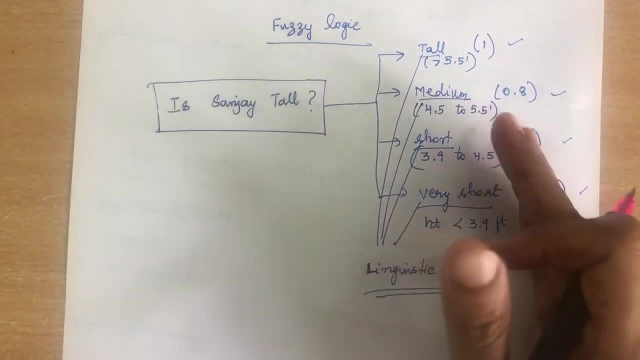 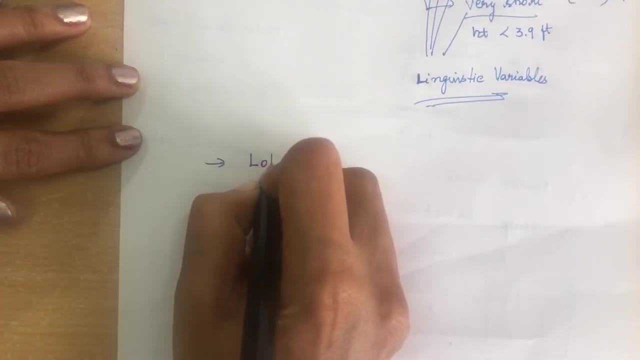 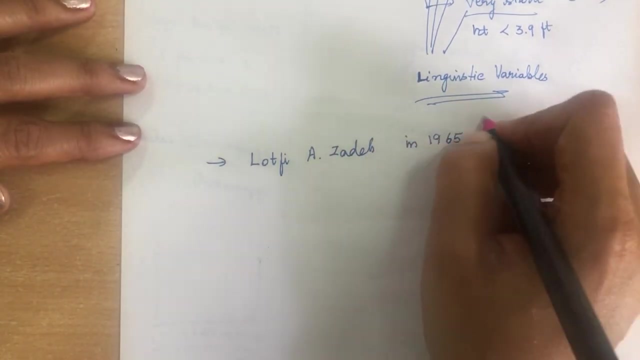 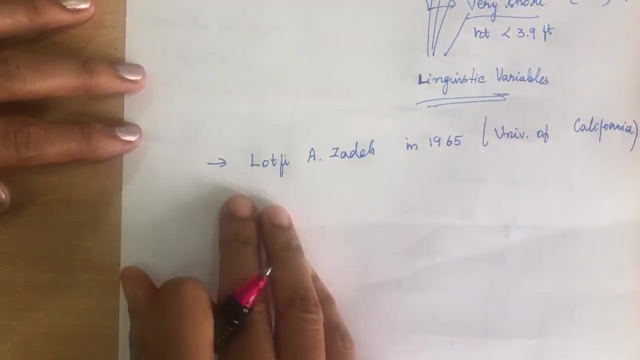 I am going to give the values for them. so this solving by this manner is called as fuzzy logic. okay, so fuzzy logic was invented by Lotfi Ajzadeh in 1965 at University of California. so he is the first. he is a person who invented fuzzy logic. okay, so why we are going for this? 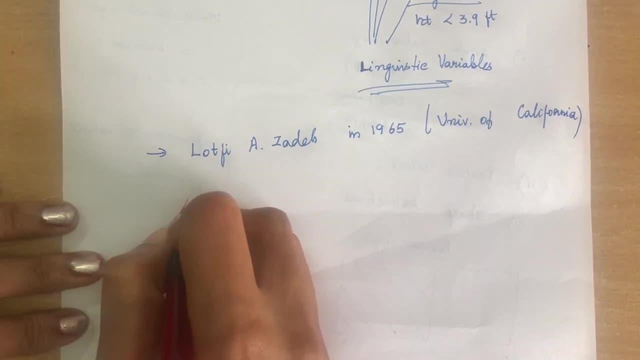 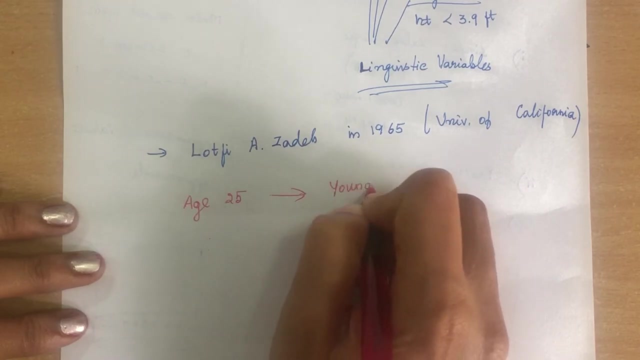 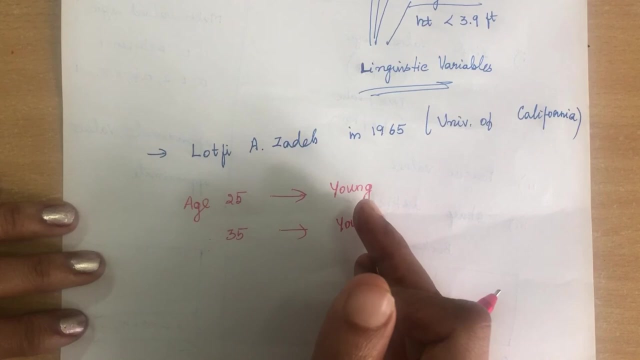 fuzzy logic. so, for example, let me tell you an example. if a person's age is 25, for some people the age 25 is feels like he is young, okay. for some others, the age 35, they will classify him as younger, okay. so we cannot able to conclude that the clear boundaries for young, young people, young age. 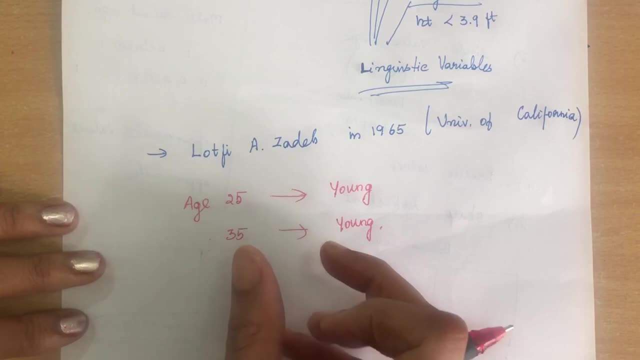 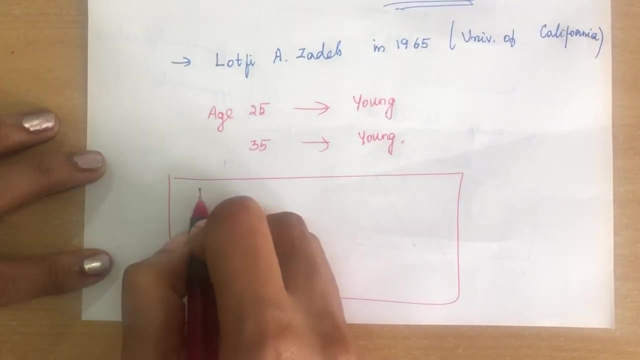 so this conclusion: this type of problems, we can solve it by solving this problem using this fuzzy logic. so what we can do is in real world problem, if you take. so, in real world problems, all the problems are not accurate, so we cannot solve it by using Boolean logic.